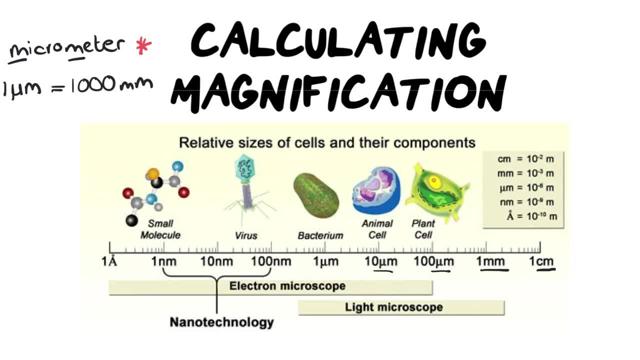 always need to convert millimeters into micrometers. So that's a rule of mathematics. You can't calculate anything in the same unit of measurement. So if you use your ruler to measure in millimeters, you must be able to convert it into micrometers. Now if we move further down, 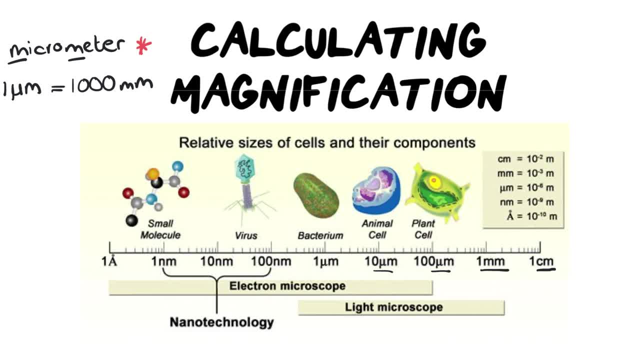 on the scale- which we're not going to do in this video, but it gets even smaller- is if we look at where the virus is and we see mm. that represents nanometers, which is incredibly small. You would need an electron microscope to see these clearly, but we're not going to go that far. We're going. 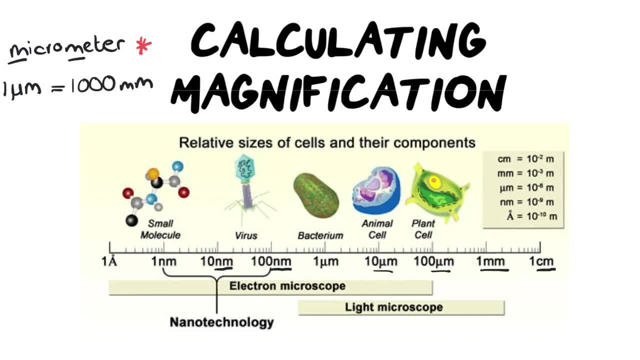 to stay just by the micrometers. Now, as a reminder, if you are new here, my grade 10 playlist is growing all year long and I'm adding new videos every week. So if you need help with life sciences for the very first time, then you should click the playlist above. now It has all the grade 10. 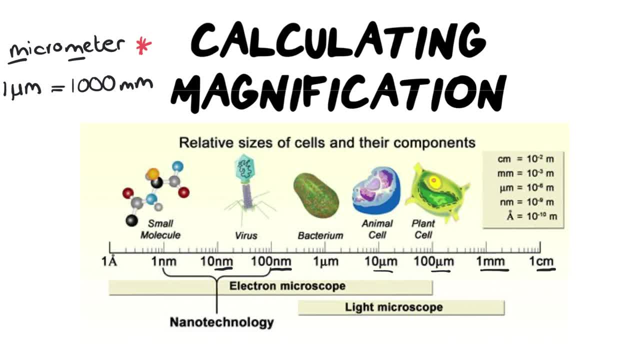 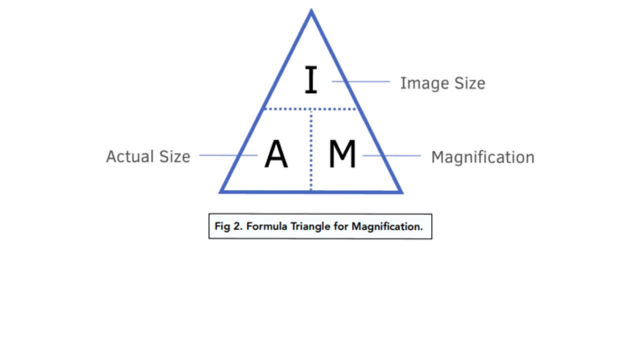 videos that are there now, and I'll be adding more all year long. So how do we actually calculate the magnification and how do we calculate the actual magnitude? Well, we've got this beautiful little pyramid over here, and this pyramid is going to tell us. 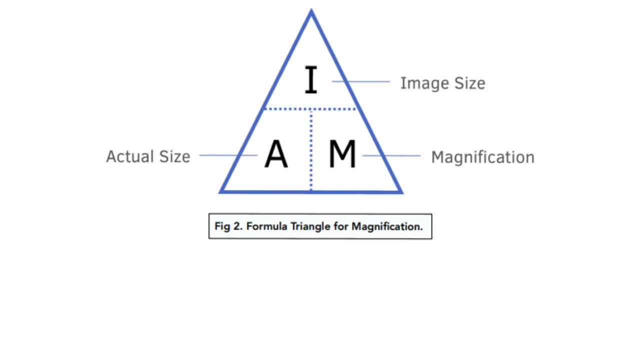 how to structure the formula to solve the missing value. So let me explain what that means. If I am looking for the actual size of something, what I'm going to do is I'm going to say A equals I over M, or image size over magnification. If, however, I'm looking for the actual size of 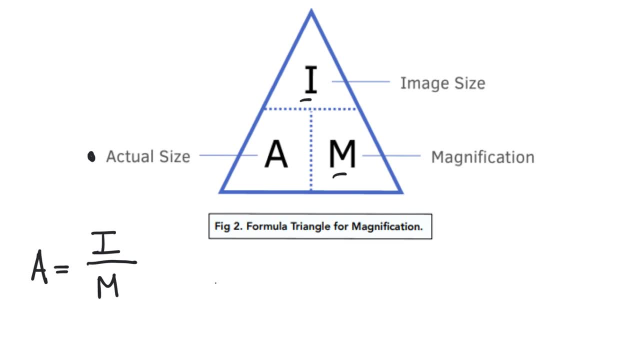 I am looking for magnification. on the other hand, I would go: M equals I over A, And the position of the letter in the pyramid will tell you how to position it in your equation. The last and final one is: if I want to calculate the image size, I would say I equals A multiplied by M, And that's. 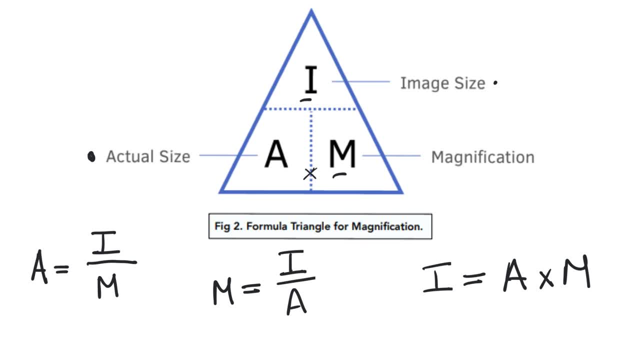 what this means here is that there's like a little invisible multiplication sign here, but as soon as there is a value above this line, it's a divide, And that's how we write out the different formula. I want you to also know that you get a mark for writing the formula, And so 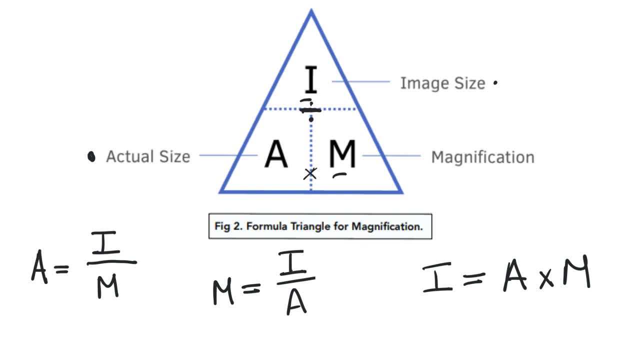 you'll be expected to do that every single time. Now let's get to the hard part right, Because I think many of us don't know what to do And we start to panic when some of these letters are missing, For example, if we are looking for the magnification, which is often the more difficult. 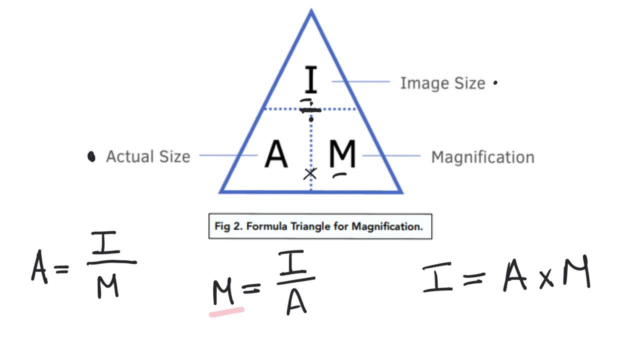 one to do, because you have to do quite a number of calculations before you get there. we go into a bit of a panic and we don't know what to do next. I'm going to show you two different examples solving two different outcomes: one for actual size and then one for magnification. 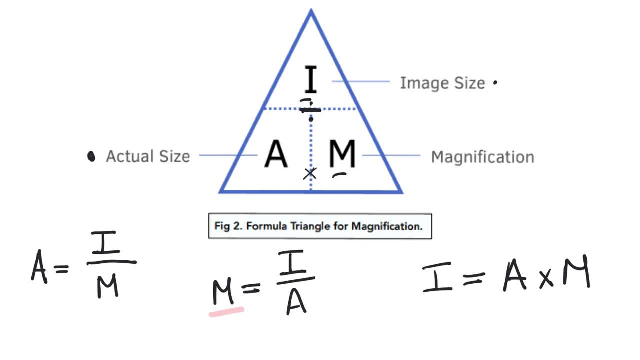 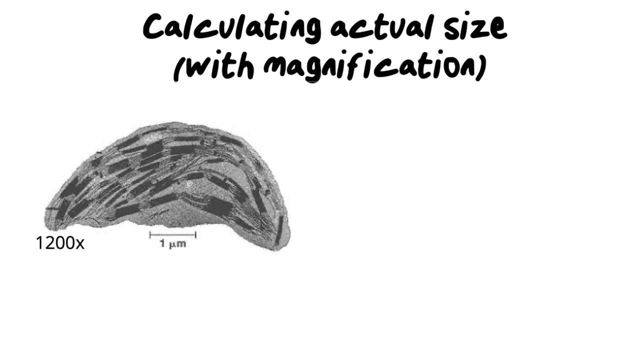 And I'm going to show you the, step by step, things that you need to do every single time to get full marks. Now let's begin with a very simple, easy example, And then we'll do a more difficult one later in the video, ones that you'll probably 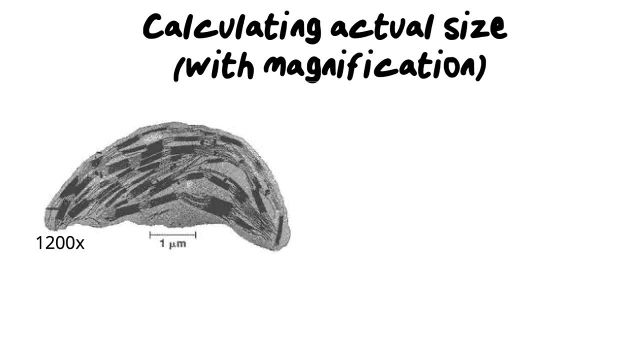 see more often in tests and exams- really the ones you actually really dread doing because they are a little bit harder. But the first thing I want you to notice is we are going to be calculating the actual size and we've been given the magnification, And the magnification is 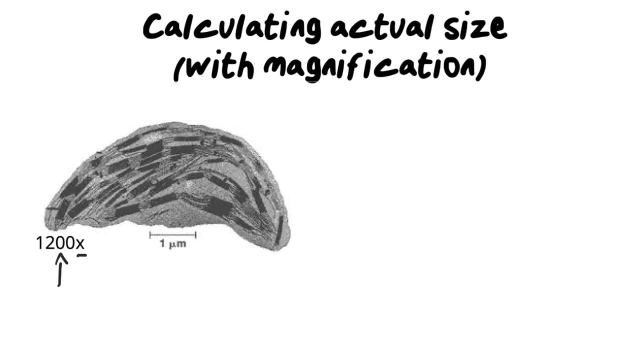 over here And I know it's the magnification because it's got this little X here. So that means this chloroplast in this micrograph has been magnified 1200 times. This other structure over here is called a scale bar, But we're going to get back to that later on. 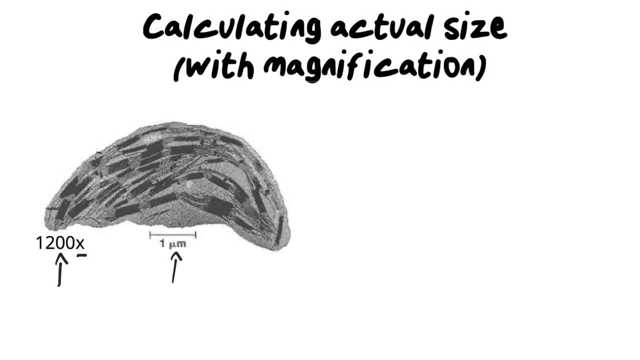 because we actually don't need it for this particular calculation, And it's really important to know when you must and mustn't use that scale bar, like when it's necessary or not. So first things first. what we always do is remember when we are calculating. 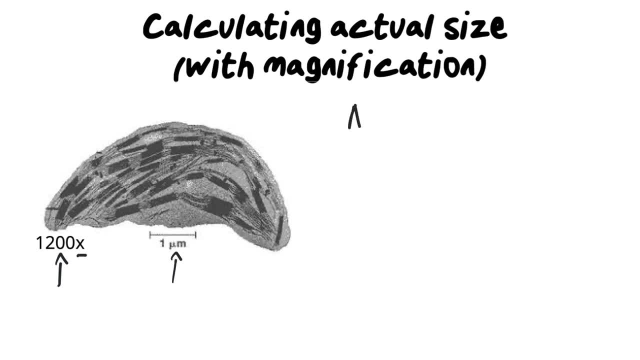 our actual size. we need to write out the formula So A equals I over M, or actual size equals image size over magnification. So let's substitute in the values that we have for now. So right now we have the magnification. So let's substitute in the values that we have for now. So right now. 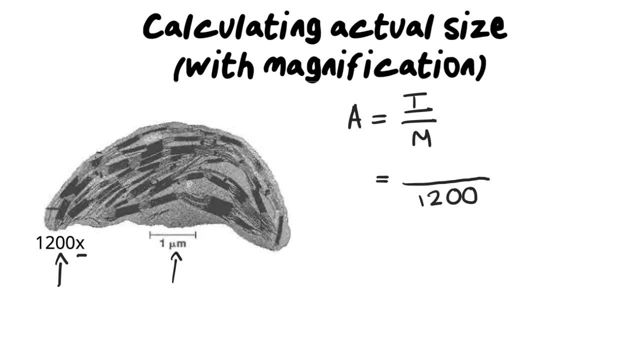 we have the magnification, which is 1200. But we need the image size. So what you're going to do is you're going to take your ruler and you're going to go to the longest or the widest part of the structure that you're trying to determine its size And you're going to go from its widest. 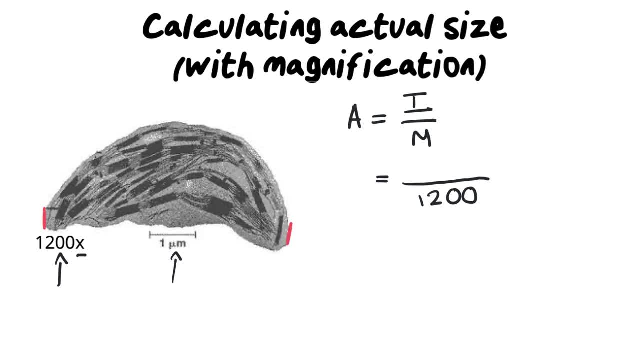 or longest point, So that would be from here to here. And then you're going to take your ruler and you are going to measure right across And you are going to then write down what it is And say: let's say, for example, it was 50 millimeters, I suggest that you measure. 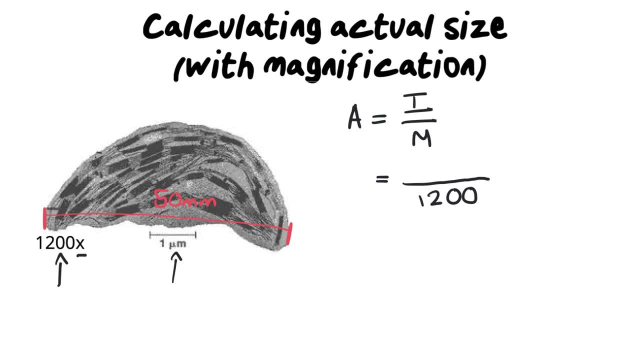 everything in millimeters, because it's going to make conversions much, much easier later on. So we're going to put 50 in our calculation And now we can use our calculator and we can divide 50 into 1200.. And we should get 0,0416.. Right Now, at this point. 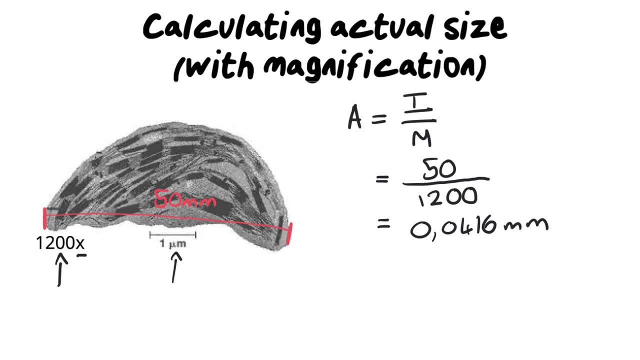 it is currently in millimeters. We need to convert it into micrometers because we are definitely not looking at this chloroplast in millimeters right now. So to do that, we actually need to times it by 1,000.. Why 1,000?? Well, remember, at the beginning of the video I told you that there. 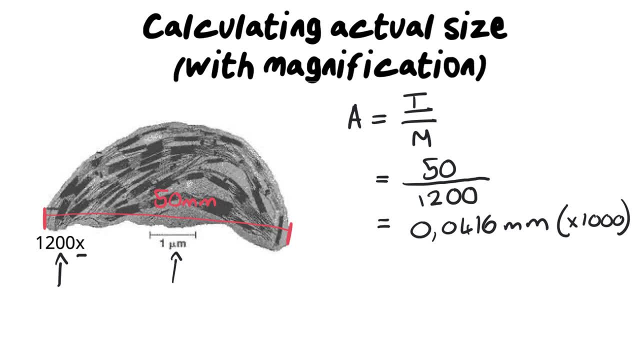 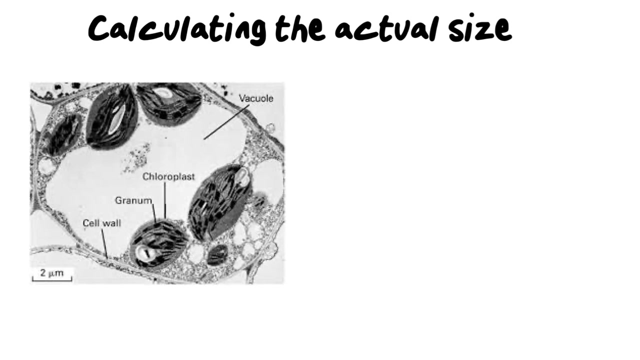 were 1,000 millimeters in one micrometer. So if we multiply it by 1,000, you should get 41,6 micrometers, And that's the simplest version that you can do. Now we come to the hard question, the one that you're dreading, because it requires you to 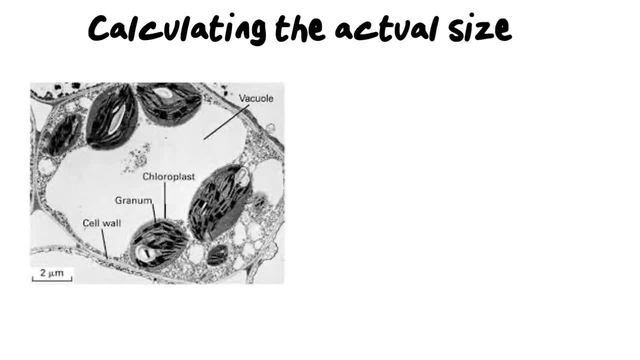 calculate two different things, And if you get the first one wrong, you will then get the rest of the question wrong. So you have to calculate the actual size, but you have not been given the magnification. Now let me show you why this is a problem. 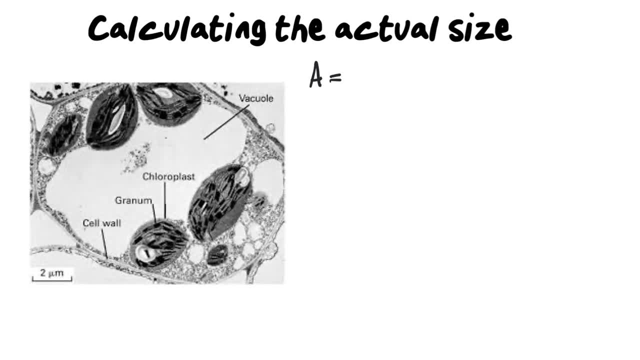 Because if we are calculating the actual size, it should be image size over magnification. Now here's the thing: If we look at this picture of a plant cell alongside here, there is no magnification identified here. So let's write out the formula for calculating. 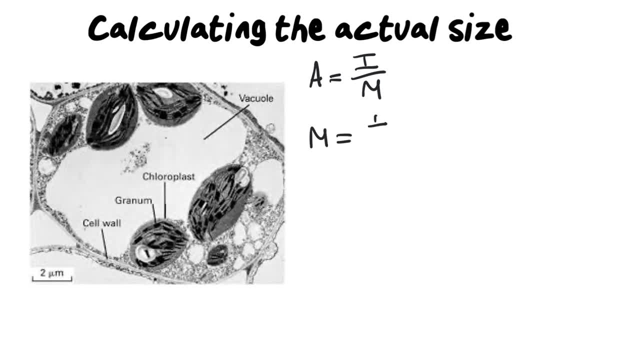 magnification. Magnification equals image size over actual size. But now we need to figure out what are we actually going to measure for those things in order to calculate the magnification. And so what I'm telling you is, when you get this kind of question where you haven't been given the 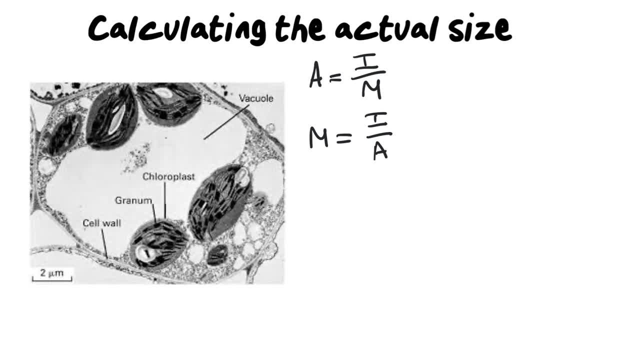 magnification. you have to start by calculating the magnification first, and then you can actually calculate the actual size of a particular structure. So let's run through the basics and let's go slowly. Now we need to start off by calculating the magnification. So we have to work. 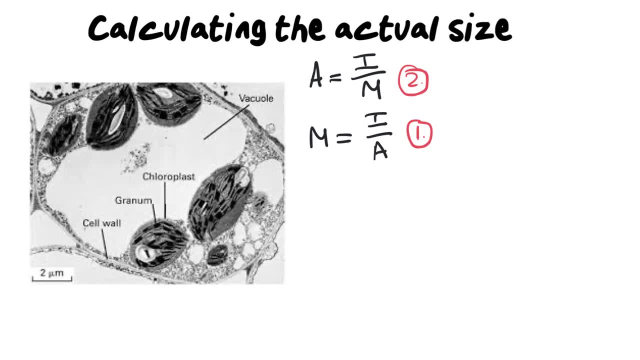 with what we've been given. And the only thing that we have been given is this scale bar right here, And that's really, really important, because what it's going to do is it's going to help us calculate the magnification. So what you need to do is you need to take your ruler and you need to. 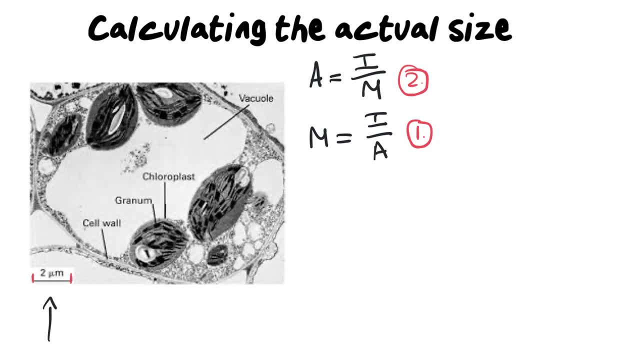 measure from this point to this point and see how you're going to calculate the magnification, How many millimeters that distance represents, Because hypothetically, if it was one millimeter, it then means that for every millimeter on this picture it will represent two micrometers in. 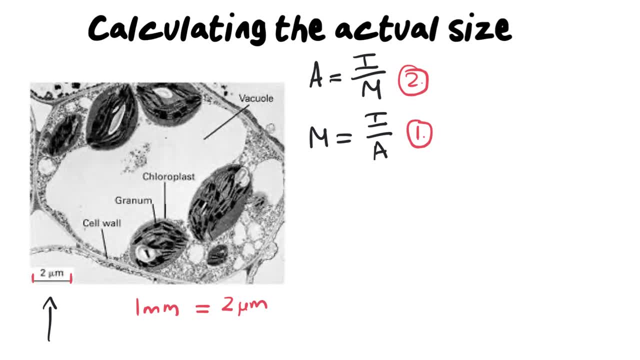 real life. That's what a scale bar does. It shows you the scale of reality that has either been shrunken down or has been magnified bigger. And that's the purpose of that scale line: It's going to tell us how to convert it and create a magnification. So let's say now: 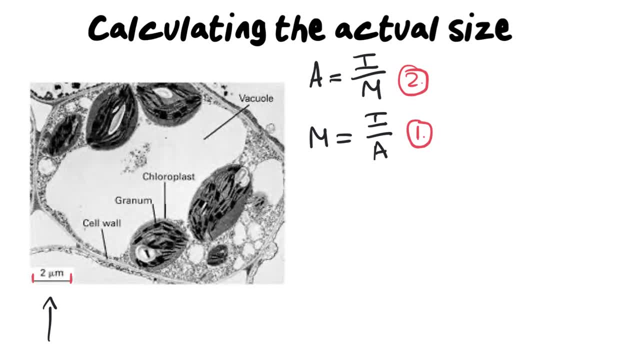 hypothetically, I'm going to measure this scale bar out And let's say that length of that scale bar is, let's say it's 21 millimeters long. Okay, Now I've got two pieces of information that I can actually substitute. I can substitute the two and the 21 to find out the. 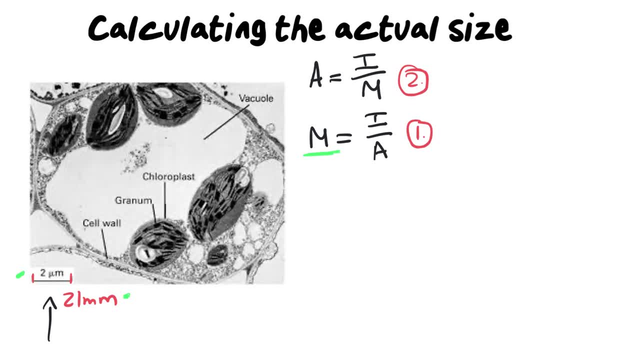 the magnification. And so this is how I'm going to do that. First things. first, I need to convert the 21 millimeters because, remember, we can't use 21 millimeters, It must be micrometers. So what we do is we go 21 times a thousand, right, Because we want to convert it, and we get now. 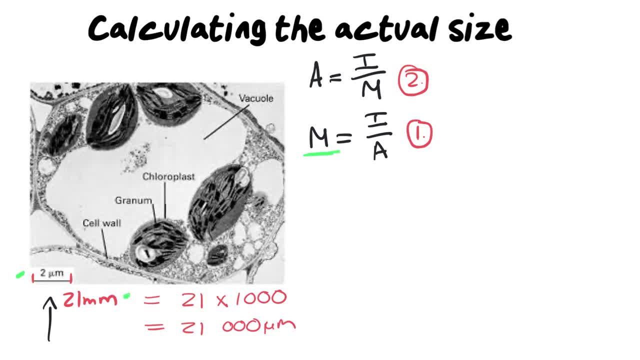 21,000 micrometers. Okay, And so now, what we're going to do is we're going to substitute these values in, because, again, we want them to be in the same units of measurement. So let's substitute them into the equation. 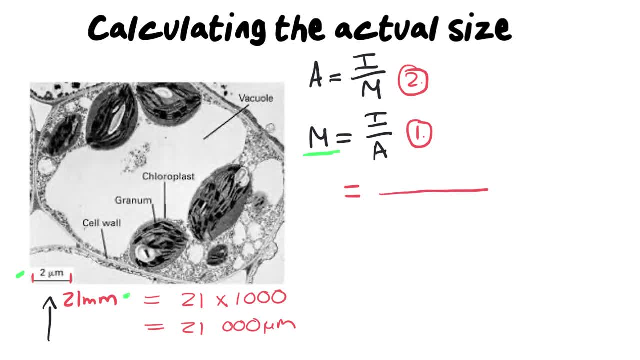 So the image size versus the actual size, which one is which? Well, the 21,000 represents our image size, The two over here represents the actual size, And it kind of makes sense, right, Because what it's saying is: 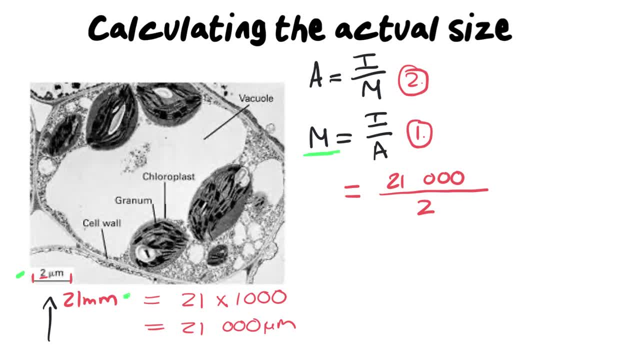 okay, scale bar. its actual size is two micrometers. Now all you need to do is put that in your calculator and we're going to go. 21,000 divided by two gives us 10,500 times. Now that we have. 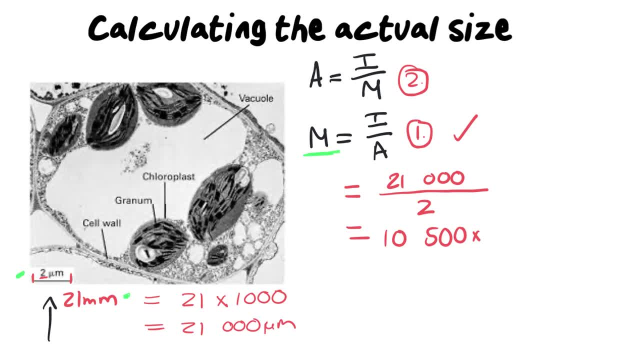 the magnification. we can now calculate the actual size of this cell that we are looking at here. And now we do as we did before. Remember we're always going to write out our formula. So: A equals I over M. We're going to substitute in: 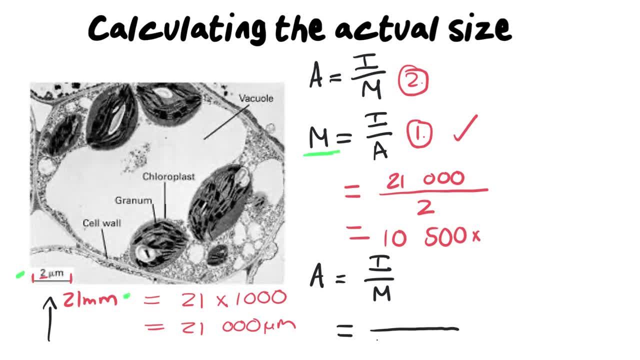 the values we have. Now, remember, the first value we definitely have is 10,500.. And now we need the image. So we go over to our plant cell and we want to look for the widest point, which I would think is over here, across to there, And we take our ruler and 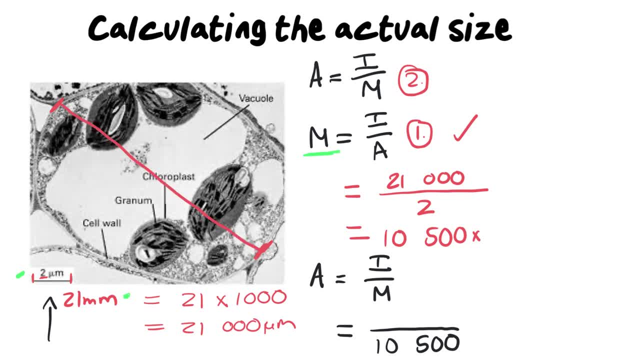 and we go straight line between these two points. And now let's say that we've measured that out And that line represents 60 millimeters. Okay, We put the 60 in, as we did before, And we use our calculator to now do some quick maths. So we say 60 divided by 10,500 times, And that will give. us what is actually quite a lot of space. So we're going to go straight line between these two points. And now we're going to go straight line between these two points And we're going to go straight line between these two points. And we're going to go straight line between these two points And we 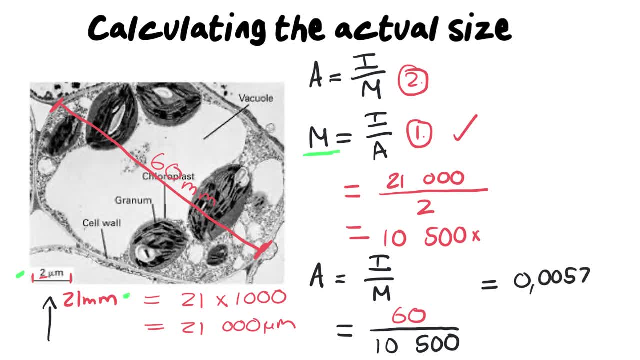 it is 0,0057.. You could potentially round it up. It's quite a long number on your calculator if you do it now, But right now this is still in millimeters Because, remember, I measured the full length of the cell as 60 millimeters. So, remember, what do we need to do? We need to. 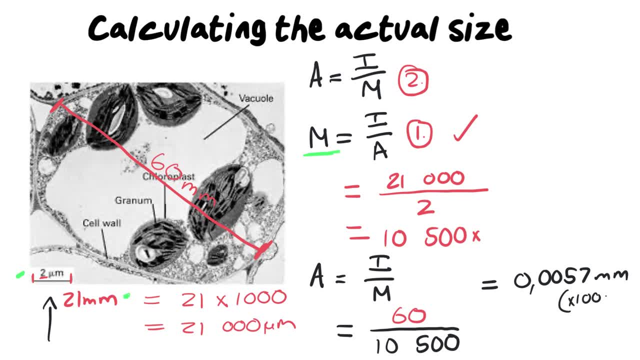 times this by 1,000 so that we can get it into micrometers, And that's exactly what I'm going to do. So I'm going to go times by 1,000 on my calculator And if we do that, we're going to. 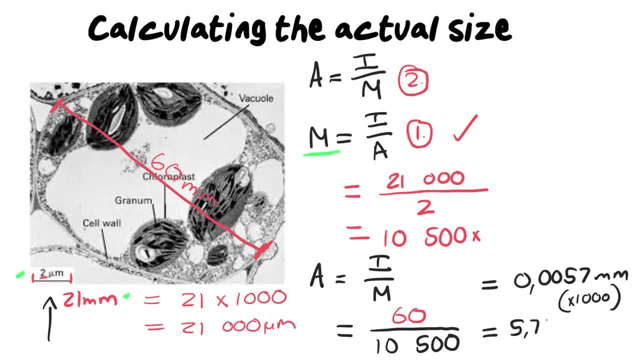 give me 5,71 micrometers. A good rule of thumb, by the way, is to always leave your answers with two decimal places. If you're unsure, then you can always round up to the two, But that's a good way. 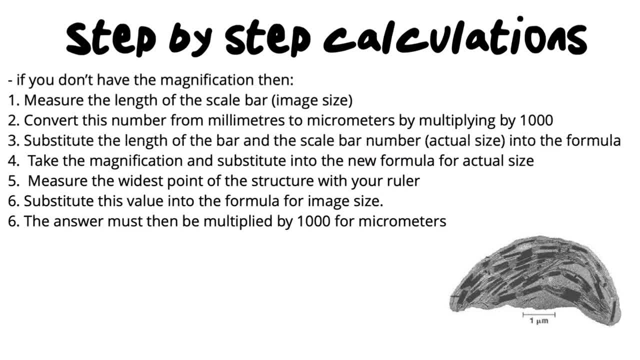 to make sure that you've given what the marker wants. Now, for those of you who prefer a more step-by-step approach, I have written out how to do the calculations step-by-step, And you can apply this to any calculation you're going to do. I'm going to do it for the more complicated one. 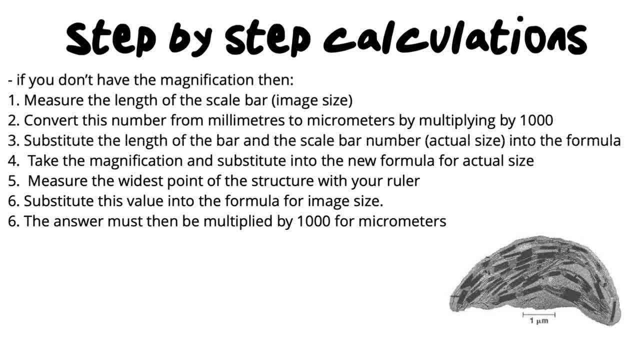 because it requires you to calculate an unknown value. As you just saw, there are two parts of the calculation, So you always have to calculate the magnification first. So you haven't been given it. So this is what we do: Measure the length of the scale bar. Remember this. over here is the 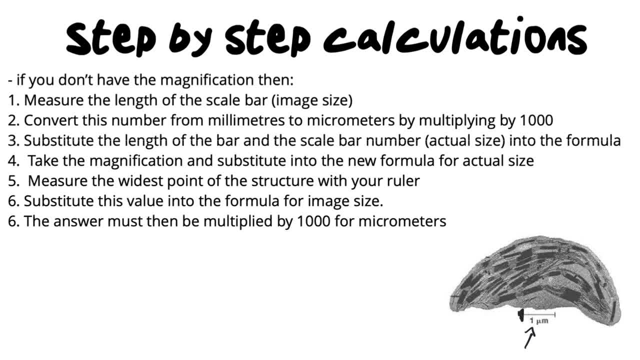 scale bar. So we're going to measure that from here to here. That is going to give us the size. You then need to convert that from millimeters to micrometers. So let's say the length of that scale bar was 20 millimeters. You need to times it by a thousand so that it can now. 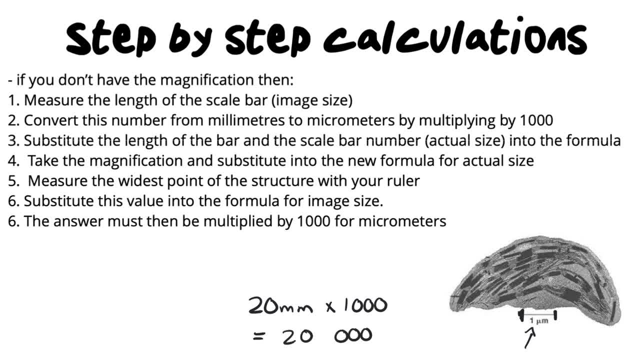 be in micrometers. Remember that's what we want. Substitute then the length of the bar, which is this value we've just calculated here, and the scale bar number or the actual size. What is the scale bar number That I'm referring to? is this number over here the one? 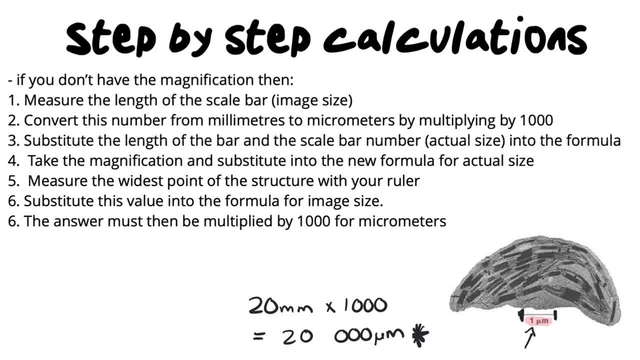 Okay, so that's the actual size. Take the magnification and substitute it into the new formula for actual size. So what that means is, once you have substituted in these two values, so the 20,000 and the one, you should then get a magnification. So 20,000 divided by one is going. 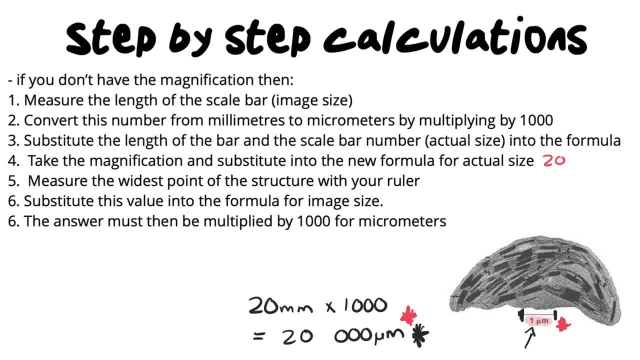 to be 20,000.. So let's say: that's the actual size. So let's say that's the actual size. So let's say now that our magnification is 20,000 times, You need to take that magnification and substitute it.